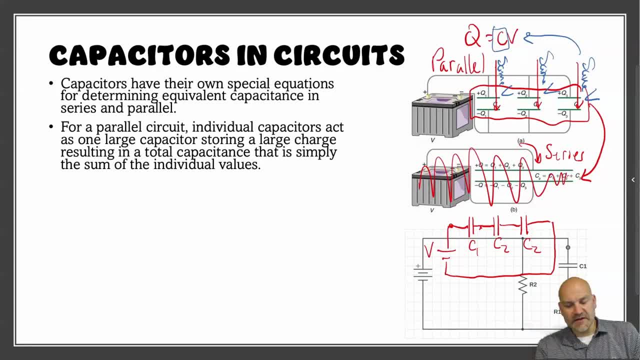 total to be the sum of those capacitors. So the equivalent capacitance in parallel is simply C1 plus C2 plus C3 plus dot dot, dot right. So all those equivalent, That's the equivalent, What is called equivalent capacitance. So for a series circuit or with: 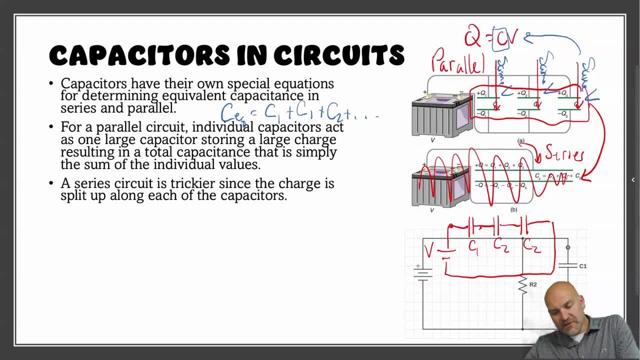 capacitors, it's a little bit trickier, okay. Again, if we look at Q equals CV, what happens is, down these Down the paths, Right, It's going to have the same charge, right? And so Q equals CV, right, And I know. 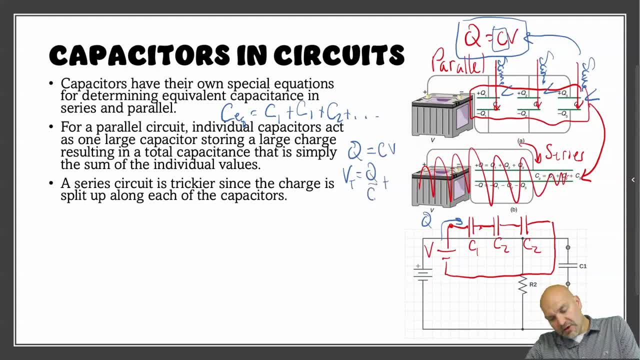 from Kierkegaard's rule that the charge, Or sorry, the voltage, has to be equal going across those capacitors. And so that tells me that Q total right Over all this, And so that tells me that the equivalent capacitance is going to be that kind of inverse looking. 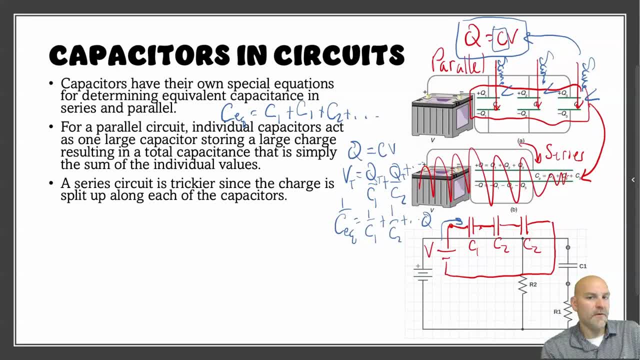 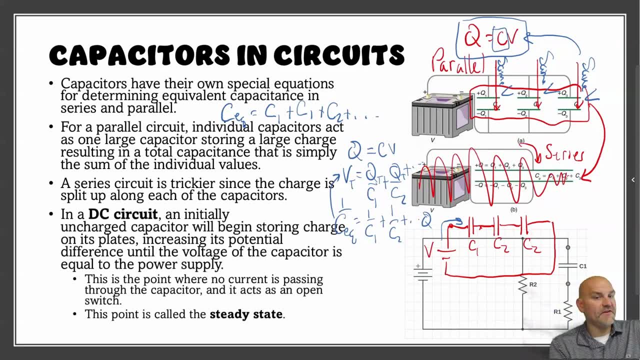 relationship that we saw with like parallel resistors. okay, And it comes from again: Q equals CV. Now in a DC circuit, an initially uncharged capacitor will begin to store charge on its plates, increasing the potential difference until the voltage of the capacitor equals the 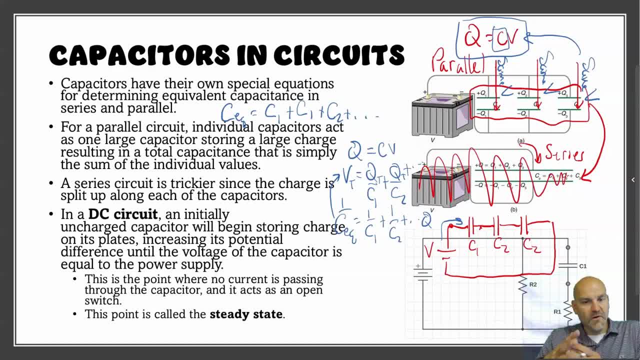 voltage of the power supply. At this point, right, there's no current that's going to be passing through the capacitor and it acts as an open switch Until you finally make the decision to discharge. And we'll get into that when we talk about the RC circuits. okay, 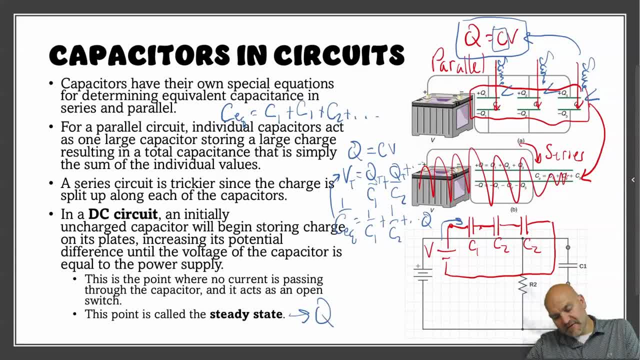 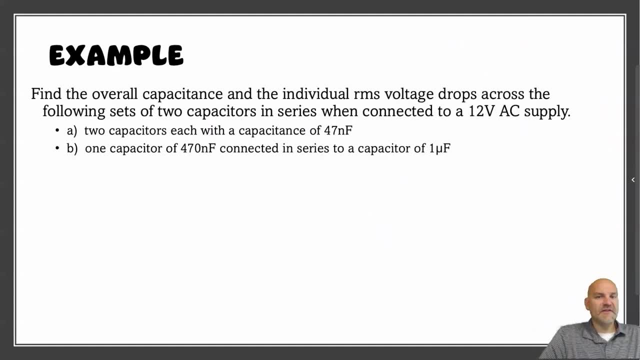 At this point it's what we call a steady state right, And so that's kind of when you get an equation like Q equals CV, right. Q equals CV tells us that it is a steady state capacitor circuit. All right, So let's look at an example problem when it comes to these capacitance. 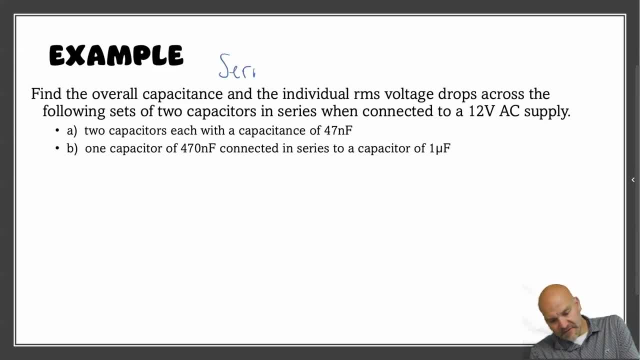 And so we're going to assume that these are going to be in series, right? So you say, find the overall capacitance And the individual RMS voltage drops across the following sets of two capacitors in series. there it is again when connected to a 12-volt alternating current supply, So A the two 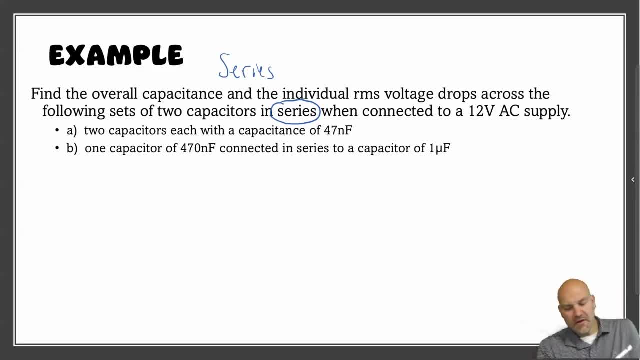 capacitors, each will have a capacitance of 47 nanofarads, which 47 nanofarads is 47 times 10 to the negative ninth farads. And then B one capacitor of 470 nanofarads, connected in series. 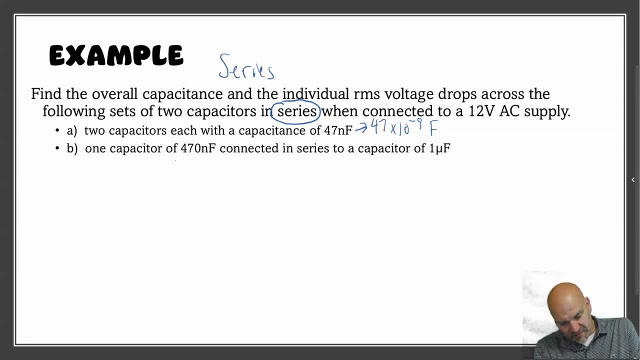 to a capacitor And then B one capacitor of 470 nanofarads connected in series to a capacitor capacitor of 1 micro farad. so this would be 470 times 10 to the negative 9th farads, and this is: 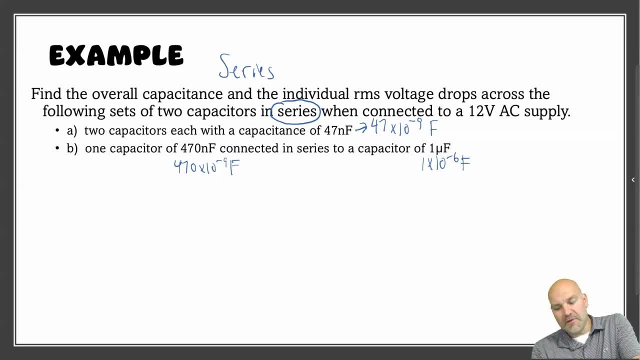 1 times 10 to the negative. 6th, farads. okay, remember, the unit for capacitance is farads, f-a-r-a-d-s right name. that through michael faraday. all right, so that's our capacitance unit. all right, so part a, i'm going to split this into two so if we want to find the equivalent resistance- because they're 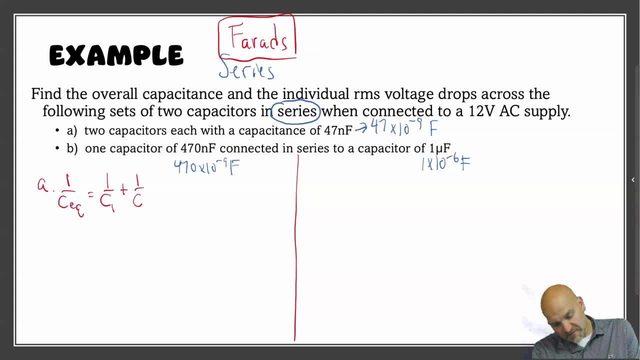 series we're going to do. 1 over cq equals 1 over c1 plus 1 over c2. this one's a little bit easy because we have the same capacitance. so 1 over 47 times 10 to the negative 9th plus 1 over 47. 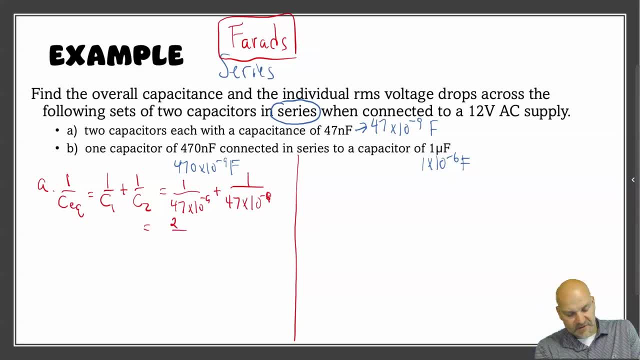 times 10 to the negative 9th, and it's going to essentially be 2 over 47 times 10 to the negative 9th. but we flip it and so we get 47 times 10 to the negative 9th over 2, or simply put: 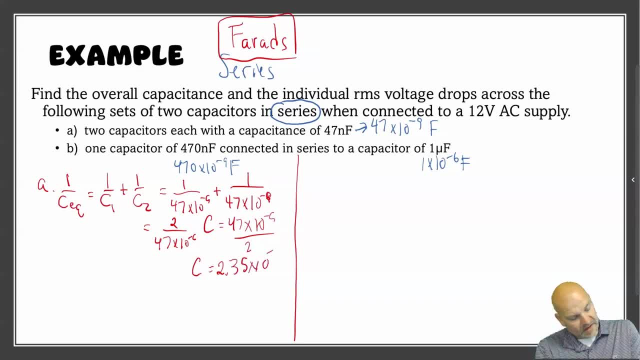 2. 35 times 10 to the negative 8th farads right. so that is my equivalent capacitance. what that then allows me to do is to solve right is to use my q equals cv to find how much charge do i have going. 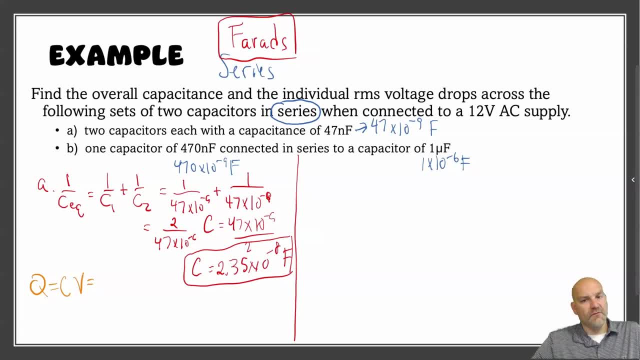 across there, right, because i can't do anything. i can't find the individual voltage until i find the, the total charge, and so it's going to be 2.35 times 10 to the negative 8th farad times 12 volts, and it's going to give me 2.82 times 10 to the negative 7. uh sorry, coulombs, right. 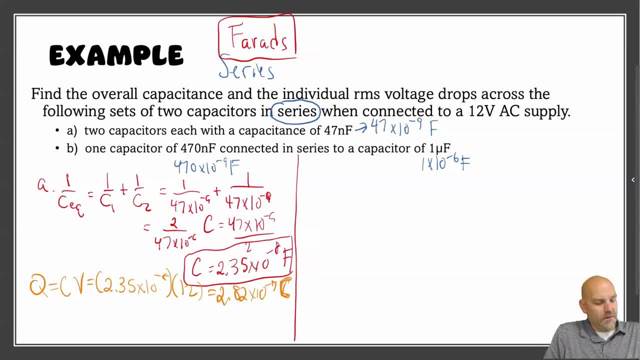 and so that's how much charge that's going across each capacitor right, and so this is actually again pretty simple. i just do q over c, equivalent, and so they're equal, they're the same capacitance. so i just find, if i find one, i find them both. 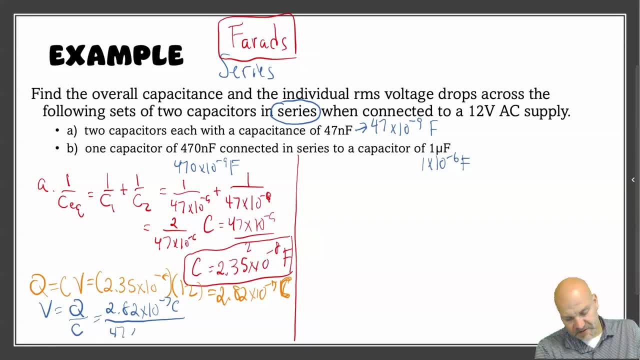 oh sorry, yep, that's charged. and then capacitance: 47 times 10 to the negative 9th farads. so voltage is a coulomb per farad. so 2.82 exponent negative 7 divided by 47 exponent negative 9, and so i get. 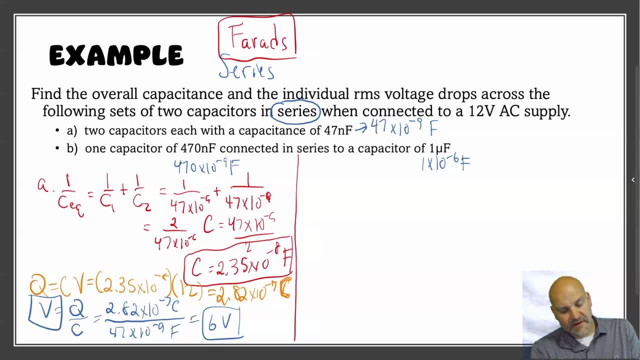 total voltage of 6 volts. is it kind of what we expected? yes, because i have two equals- uh, two equal- capacitors with 12 volts. they should, it should split evenly, all right. so now let's do part b. now we have one capacitor at 407 470 nanofarads and 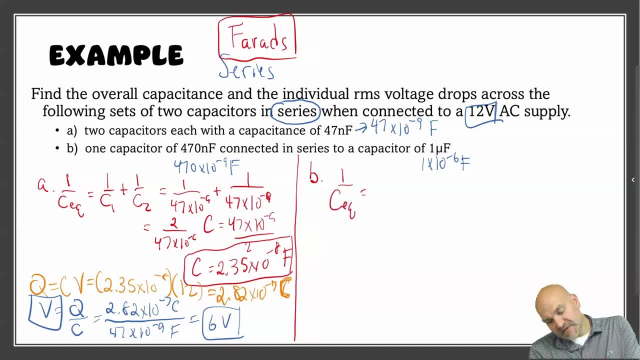 another at one microfarad. so again, equivalent resistance, one over c1 plus one over c2, so one over 470 times 10 to the negative 9th, plus one over one times 10 to the negative 6th. okay, this will give me, um, uh, you know something over. 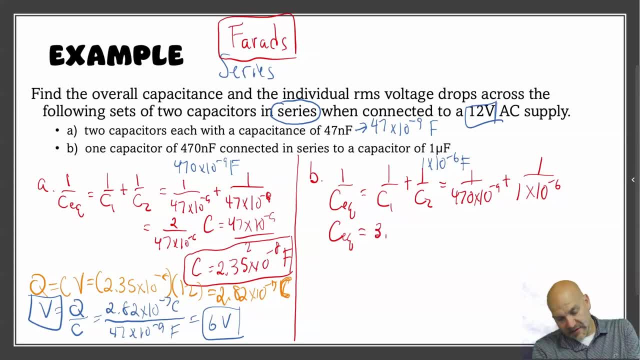 times 10 to the negative- something right. and then, when i flip it, i get 3.19 times 10 to the negative. 7th farads, which is 319 nanofarads, whichever one you want to call it. so there's my equivalent. 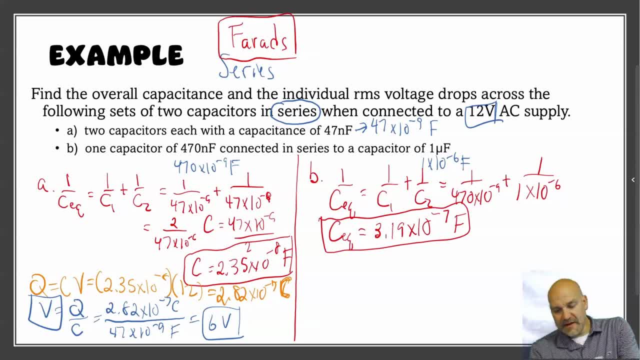 resist or equivalent capacitance. now i take that number again: q equals cv, and so i'm going to solve this, for so i have. 3.19 times 10 to the negative 7th, and so i'm going to solve this, for so i have. 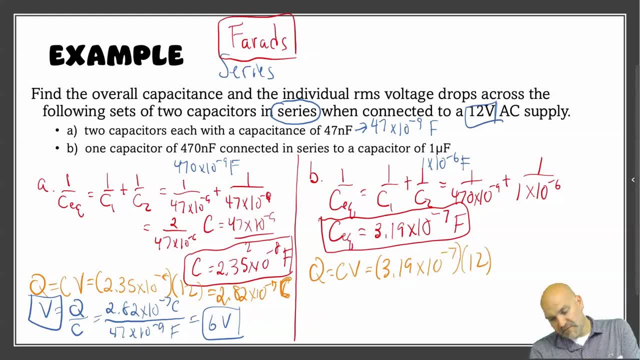 3.19 times 10 to the negative 7th times 12 again. this step here- what's in orange- allows me to find the total charge that is going to be stored on those capacitors, and so i get an equivalent, or, sorry, a total charge of 3.84. 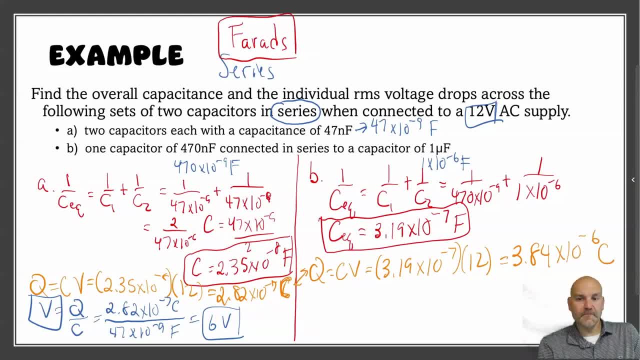 times 10 to the negative six coulombs. and now i can find each individual right um voltage. so v equals q over c, so 3.84 times 10 to the negative 6 coulombs, over 470 times 10 to the negative 9. 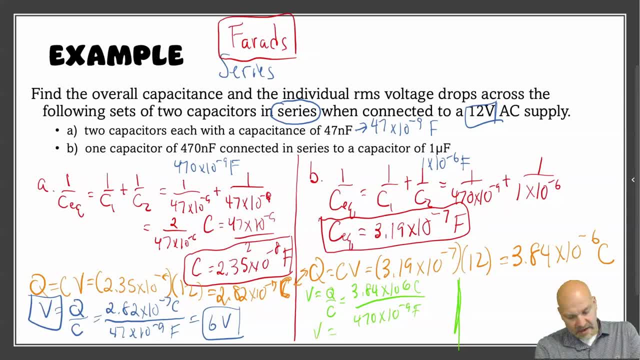 farads, and so that gives me a voltage of 8.2 volts. and now i find the next one again: q over c. so 3.84 times 10 to the negative 6, divided by 1 times 10 to the negative 6.